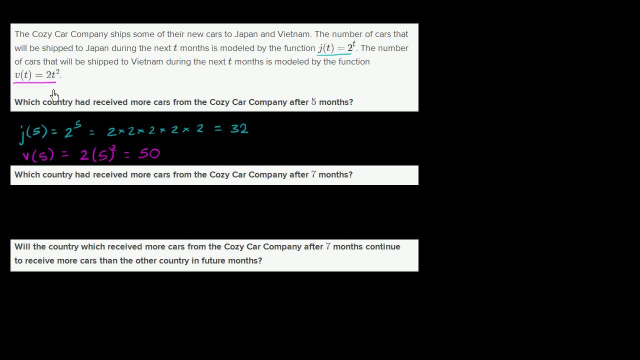 they're going to receive after t months. after five months, Vietnam is going to receive, Vietnam is going to receive more cars. So I guess the answer to that is: Vietnam, Vietnam And Japan will have received more cars after five months. Which country had received more cars? 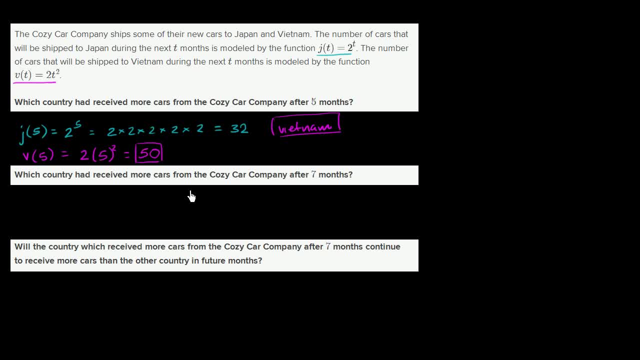 from the Cozy Car Company or will have received more cars after seven months. So once again, let's try this out. J of seven is equal to two to the seventh power. Let's see, two to the sixth is going to be 32 times. 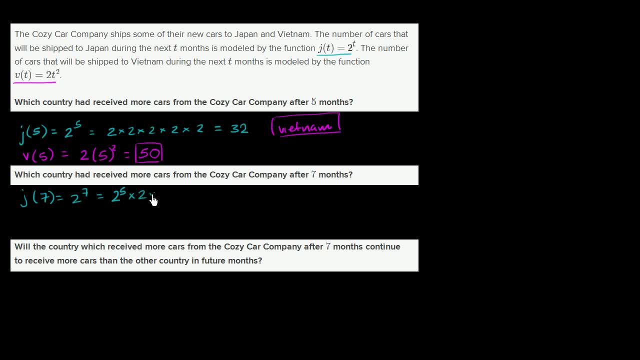 this is. we can view this as two to the fifth times two times two, which is going to be equal to. this is going to be equal to two times two times two, equal to 32 times four, which is 128 cars. 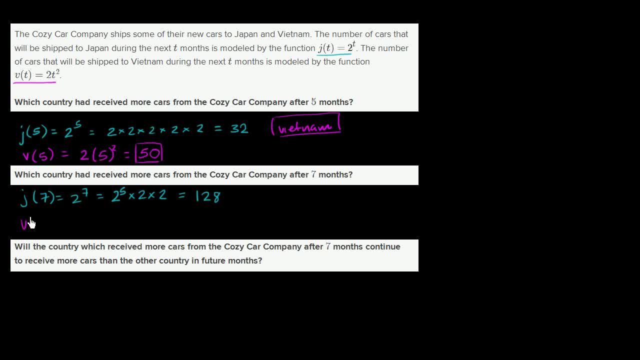 after seven months, will have gone to Japan And to Vietnam. V of seven is going to be equal to two times seven squared. so that's equal to two times 49,, which is equal to 98 cars. So after seven months, Japan would have received more cars. 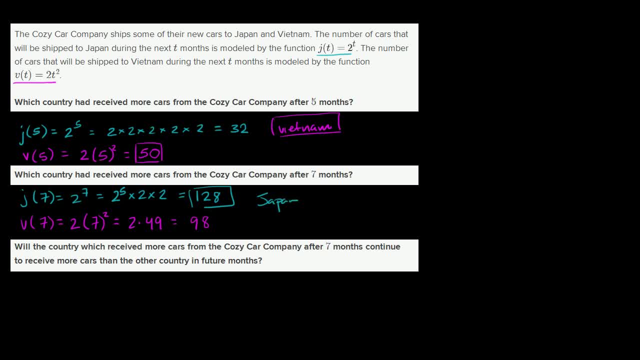 So Japan, Japan will have received more cars after after seven months, And so this is interesting. We see that the exponential function, notice, where you have the t as the exponent, that, although it might start off a little bit slower than this, what's essentially a quadratic function, 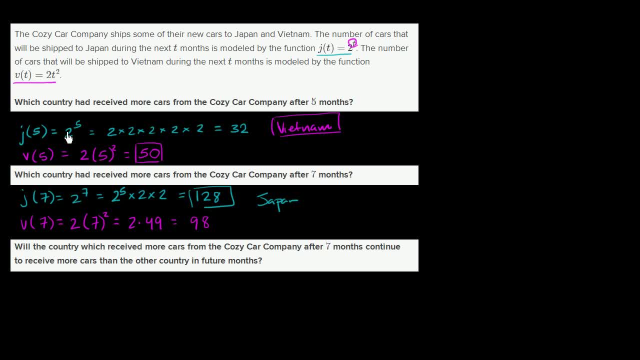 when you have something squared, it starts off slower. After five months you would have shipped fewer cars than using the quadratic model right over here. But then it more than catches up and it starts to increase at a faster and faster rate. 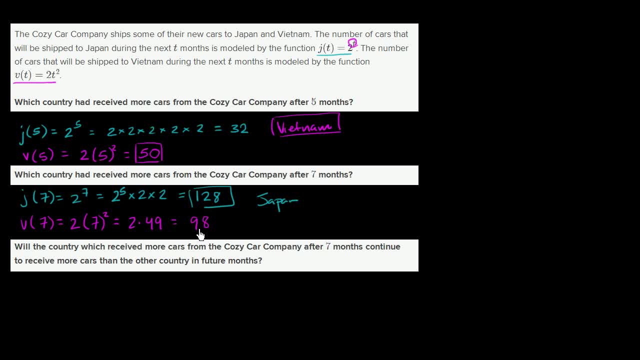 And even by seven months, it's able to pass up the quadratic function. Which country will have received more cars from the Cozy Car Company after? will the country which received more cars from the Cozy Car Company after seven months continue to receive more cars than the other country? 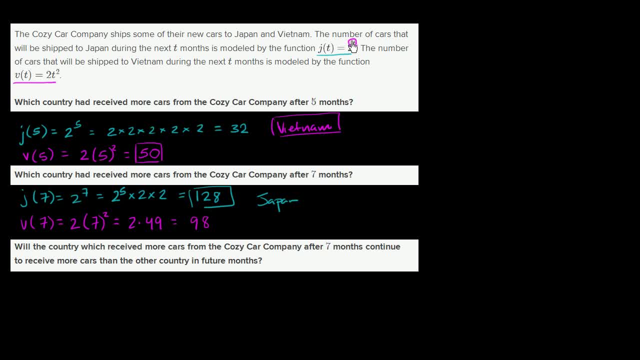 in future months? Yeah, absolutely. Once the exponential function passes up the quadratic function, it just goes faster, it just keeps increasing at a faster and faster rate. And you could see that, if we wanted to do, if we wanted to compare eight months, so J of eight, this is the exponential function. 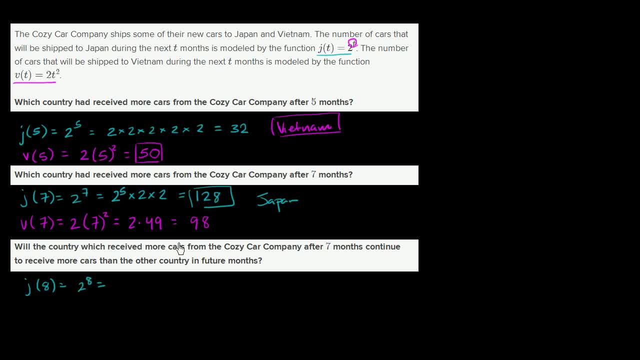 this would be two to the eighth power, which would be this times two, they'd get 256 cars and V of eight. V of eight is going to be two times eight squared, which is two times 64, which is 128.. 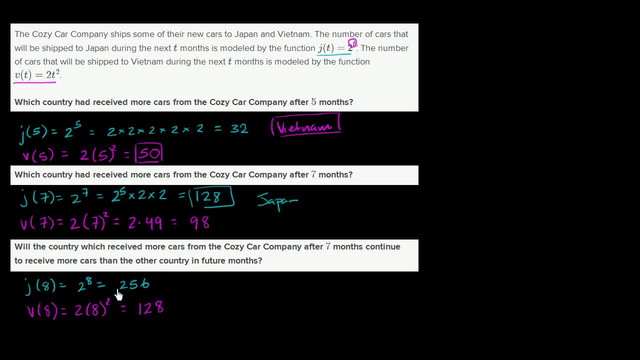 So notice now: now we would have shipped twice as much to Japan as Vietnam, Which isn't what the case right over here. We shipped more to Japan than Vietnam, but not twice as much. And we could keep going. We could. if you want, you could go to J of. 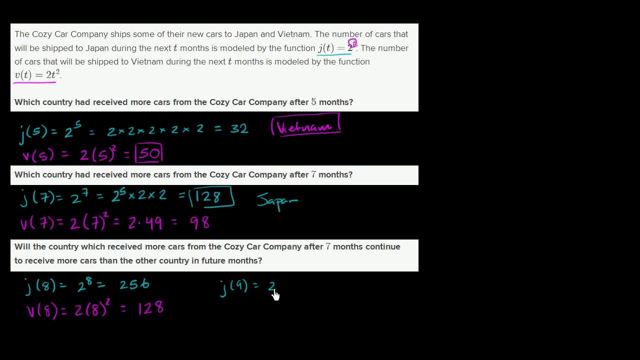 you could go to J. J of 9 is 2 to the 9th power, which is going to be 256 times 2, or 512 cars, While V of 9 is going to be 2 times 9 squared, which is 2 times 81,, which is 162.. 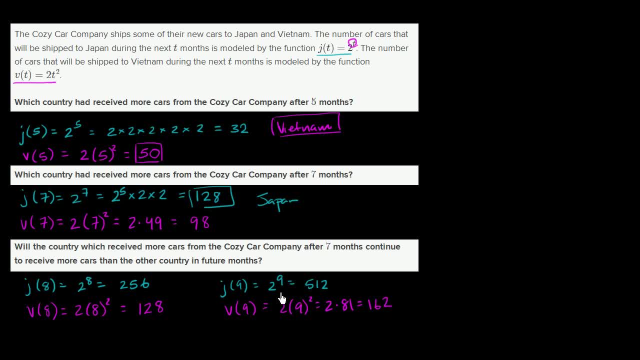 So now it's way more than double, actually more than triple. So you see that once you get past those initial few months, the exponential function is increasing at a much, much, much faster rate And we can actually visualize it. Let's actually get out a graphing calculator to visualize these two things. 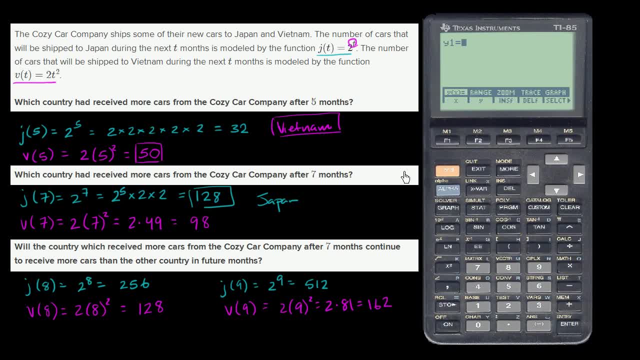 to see how that is happening, So let's graph it. So the first one: let me graph the exponential. So 2 to the- well, I'll just say x power. We'll say x is our independent variable here. So 2 to the x power. 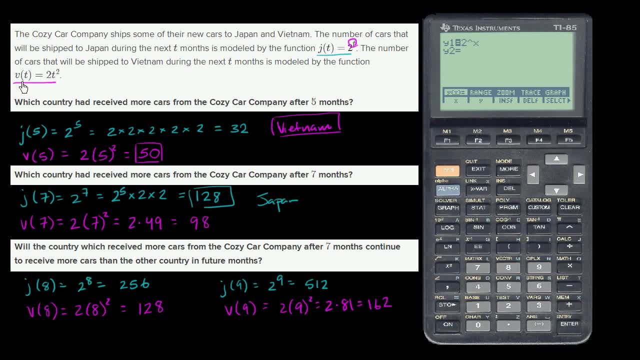 And then let's do the quadratic one. This is y2, so it'll be V of 2.. Let's say 2 times x squared. 2 times x squared. Now let me set the range. So let me set the range here. 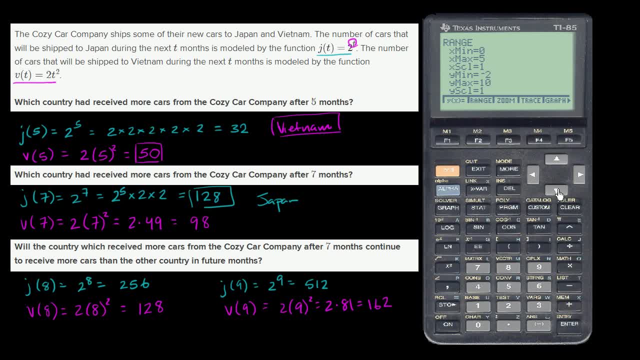 So let's see, Let's say x starts at 0. And then let's say it goes up to. let's say it goes up to 10.. Let's say it goes up to 10.. The x scale could be 1.. 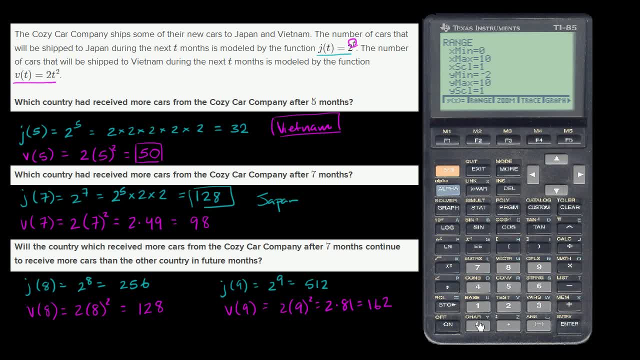 Yeah, x scale could be 1.. Now y minimum: let's say: we'll start at 0.. And then y max: we'll say: let's go to 1,000.. Let's go to 1,000.. Let's make the y scale 100.. 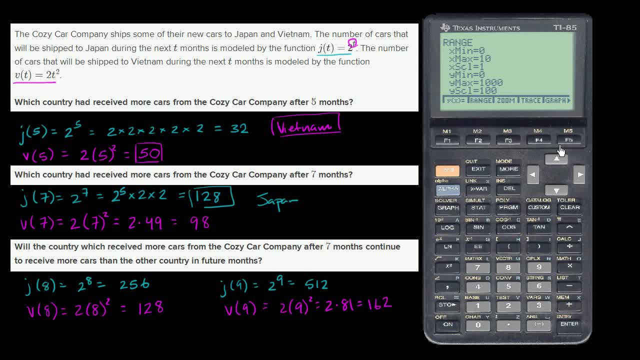 100.. And now I think we're ready to graph, So let's graph this, Let's see what happens. So it's munching on things, So that right over there that's the exponential, And then there you see, right over there you have the quadratic. 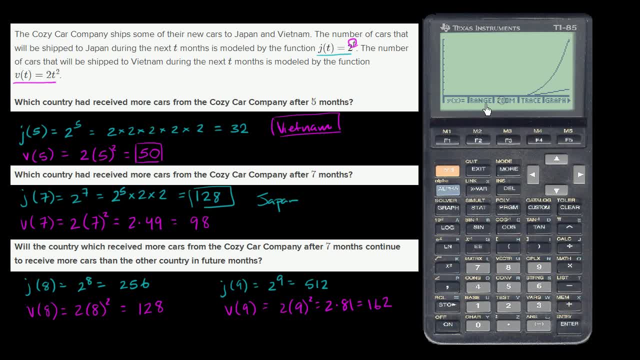 And actually let me zoom in a little bit on this so that we can see where they pass. Actually, let me zoom in a little bit on this, So I'll do it with a box So that we can really see, We can see where they pass. 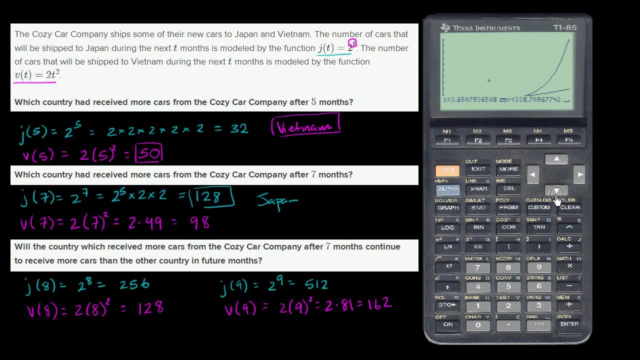 Or attempt to see where they pass each other up. So I'm going to start there. I'm going to make my box, let's see go whoops. It's weird using a calculator on a computer like this, But you see, you definitely see even what we've already graphed. 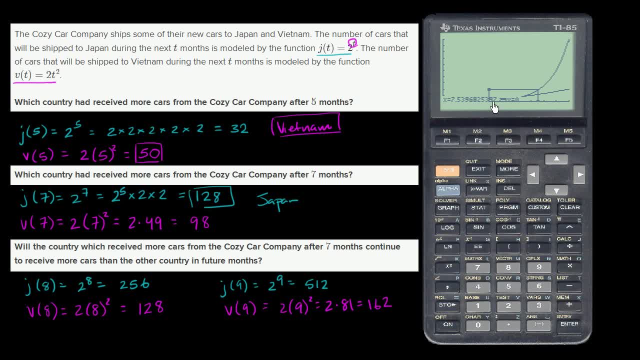 that the exponential really just starts to shoot up, while the quadratic is just going well. it's still increasing at a decent pace, but nowhere near as fast, And the difference is becoming more and more pronounced as time increases. So let me just make sure that's as low as that. 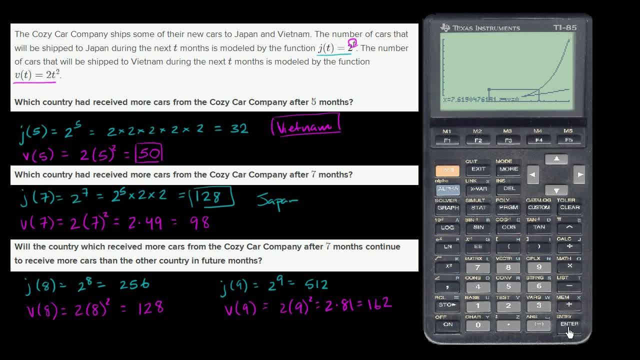 And let's graph over in this range right over here. So let's see That right over there that's the exponential function, That's 2 to the t power, And then that right over there is the quadratic. So you see, you definitely see that earlier on. 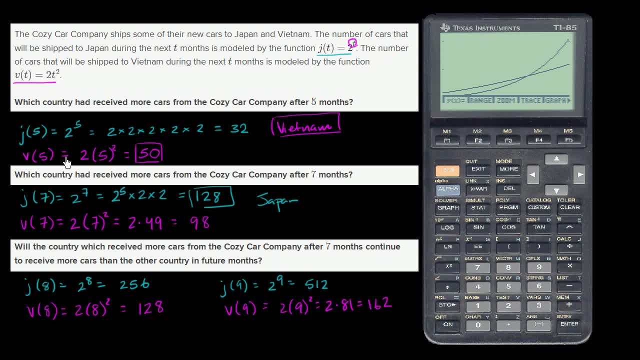 the quadratic has higher values And you see that right over here. After five months we shipped more cars to Vietnam, But then the exponential passes it up and then just keeps shooting faster at an ever-increasing pace. 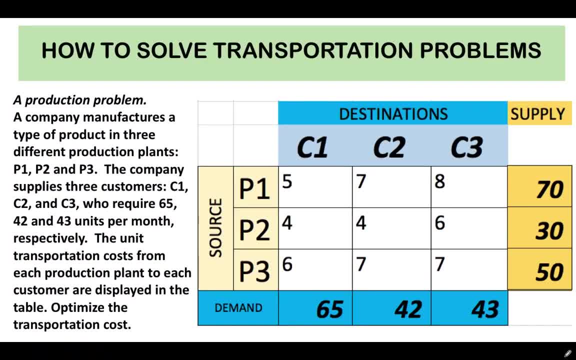 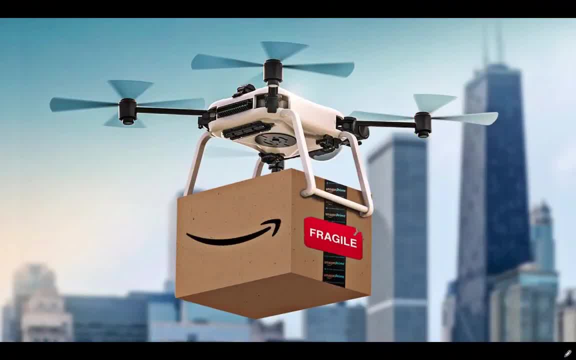 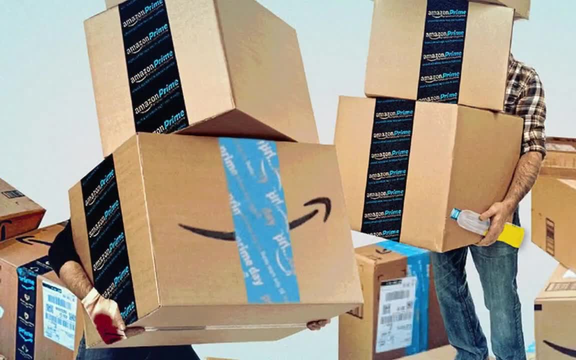 Hello everyone, my name is Lando Asisten, assisting you with another math video. In today's fast-moving world, finding a mathematical solution for transporting merchandise from one place to another and for allocating resources from several production facilities to the customer's location that minimizes time and cost is an important field. 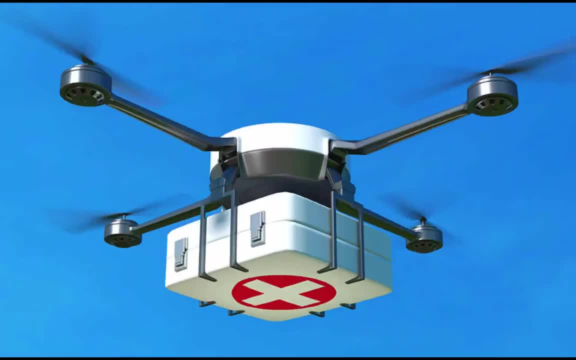 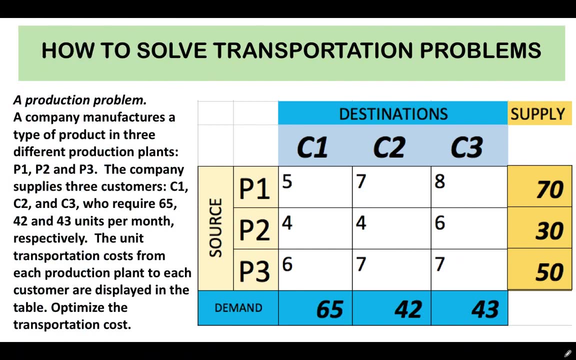 of mathematical application. In today's lesson we are going to talk about how to solve transportation problems, But before that a little background about transportation theory In mathematics and economics. transportation theory or transport theory is a name given to the study of optimal.